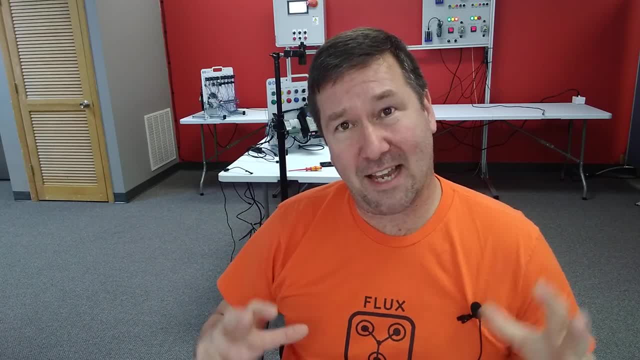 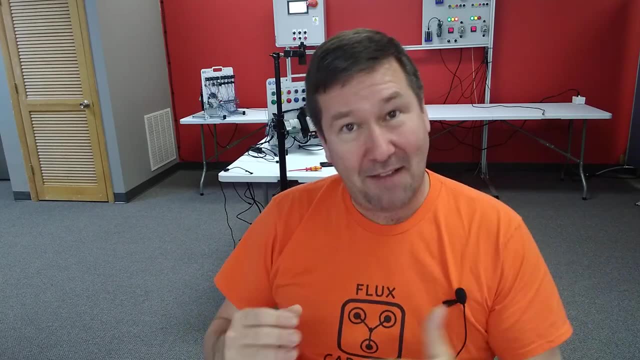 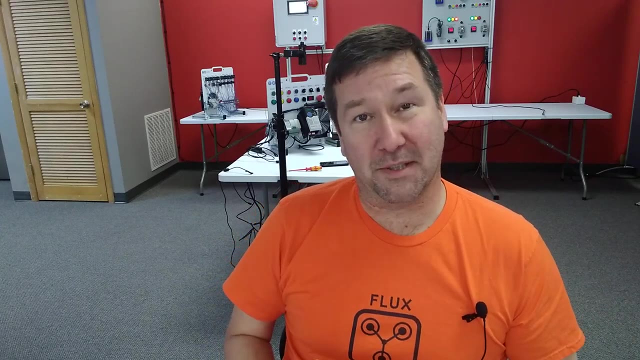 gets me excited because when you're on the outside looking in at our industry, similar to a lot of industries, it can seem impossible to navigate to get into it and it really is easier than it appears. But there are some critical moments and I do believe these first few steps to getting into 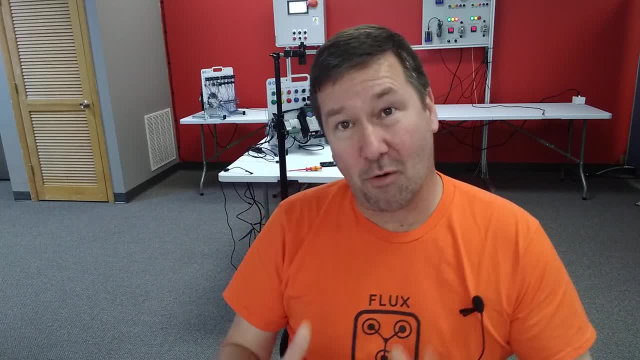 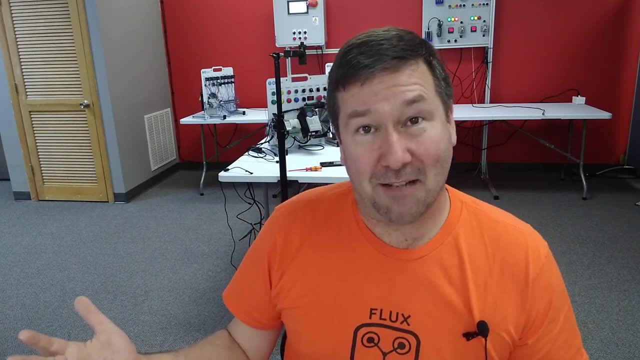 it have a lot to do with whether you will succeed or fail at your journey. If I had to break it down, oh, let's say, to three steps, then the first step is determining what brand people are going to be using and what brand they're going to be using for their product. 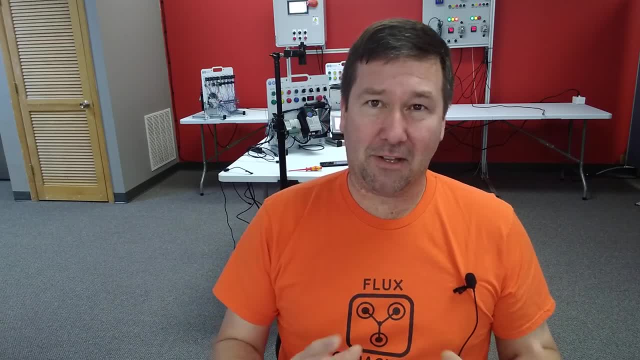 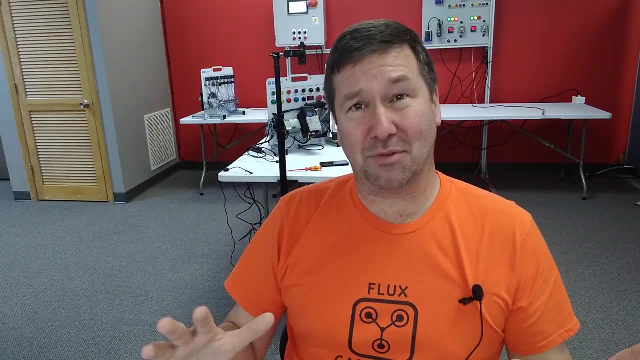 The second step is determining what kind of PLC that you want to learn, because I disagree with a lot of people on this. A lot of people will tell you that you should get a broad knowledge of a lot of PLCs, and I see schools do this and I really discourage them from it because you know they'll set up for a little bit. 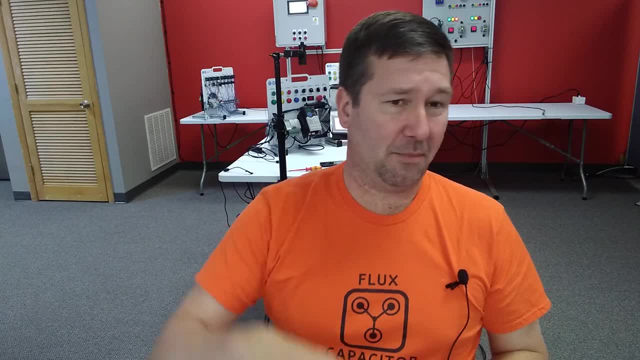 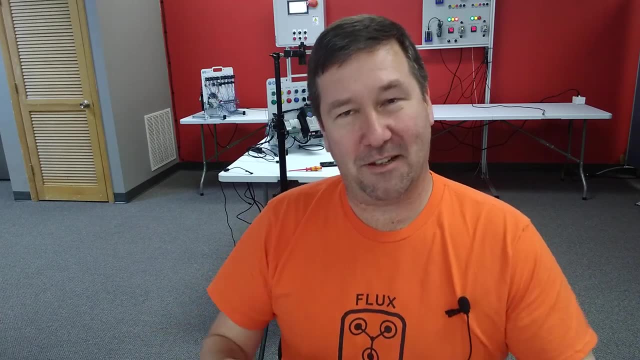 of Allen Bradley and a little bit of Omron, a little bit of Siemens and a little bit of Mitsubishi and a little bit of Automation Direct and they'll have the students kind of skip across the PLCs throughout the semester. But in the end 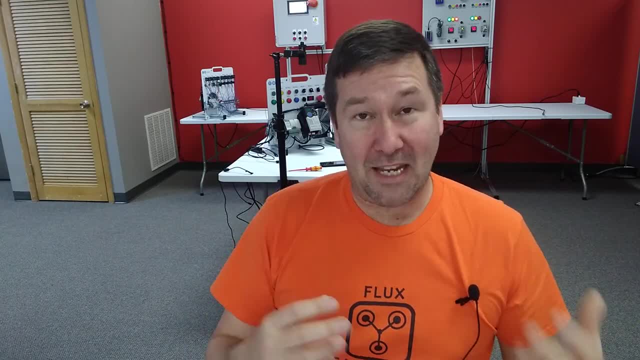 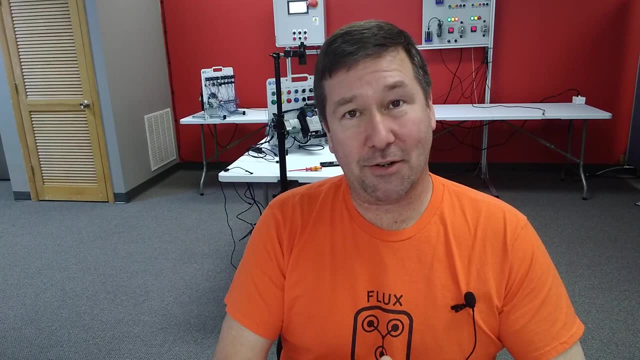 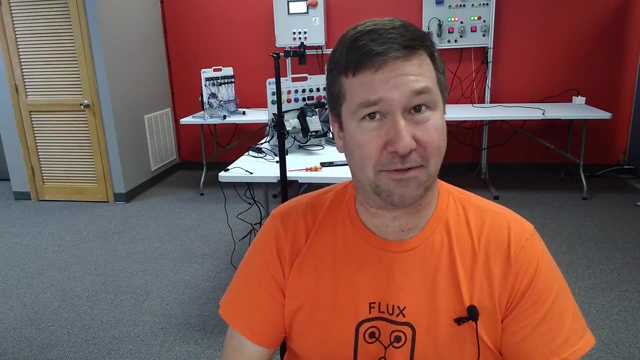 they don't have an in-depth knowledge of any of them. So I really do believe that you should choose one and learn it inside and out. I mean, learn every single instruction, every single aspect of it, every single little feature of it, how to do all the little things- and then you're going to 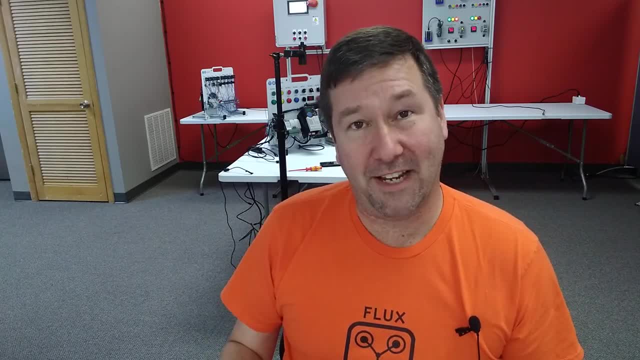 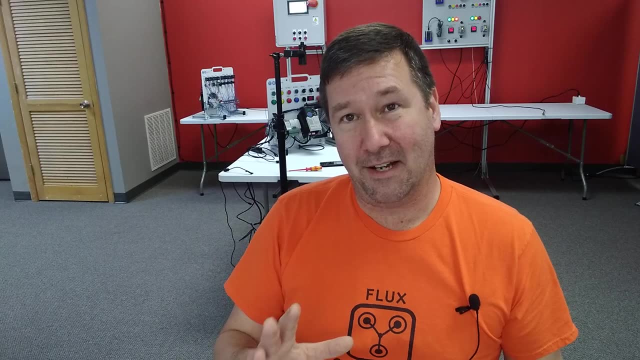 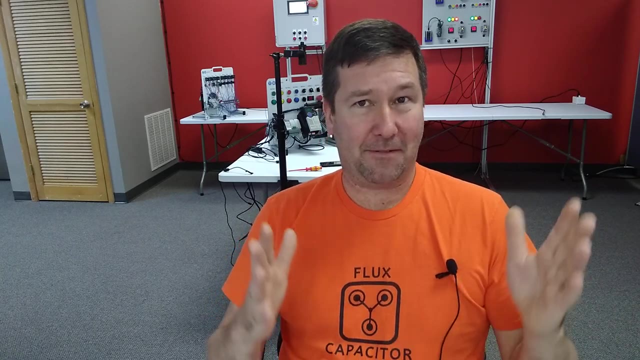 find that once you have that really strong foundation, you can jump from Allen Bradley to Siemens, to Omron if necessary. But especially starting out, you shouldn't be intending on doing that. You should have a path that will probably keep you on one particular PLC, and that's why 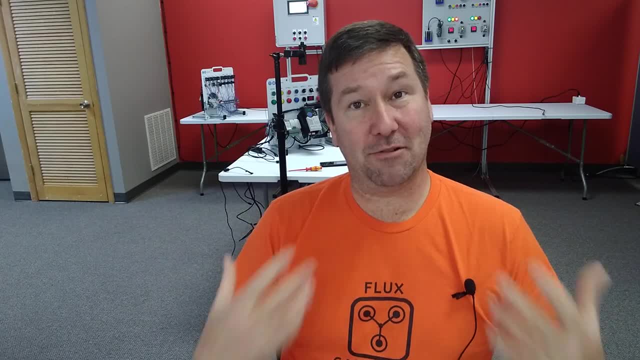 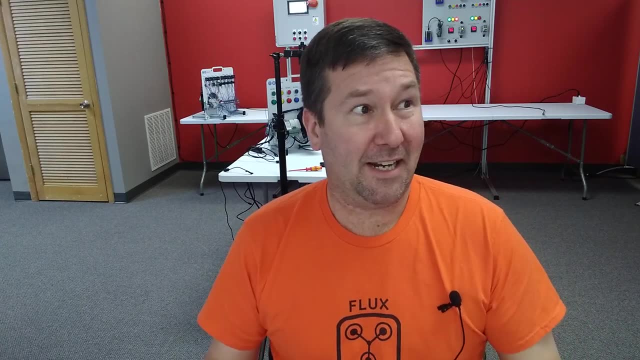 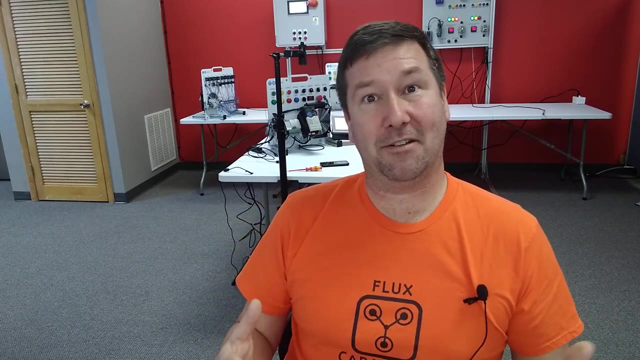 really, when it comes to what brand I recommend that you learn on, it is going to be the brand that is the most popular in your area. Now do not go to your local supply house and say, hey, what is the most popular around here? Because they're going to tell you the PLC they sell is. So you need 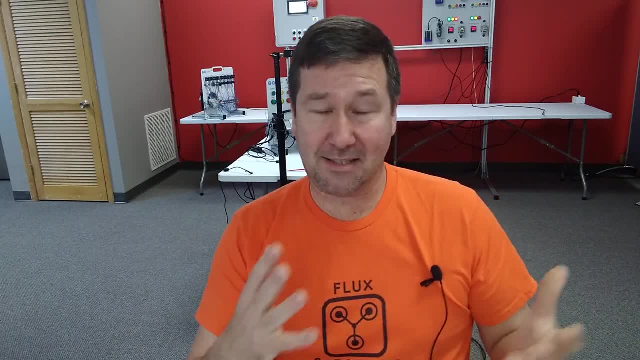 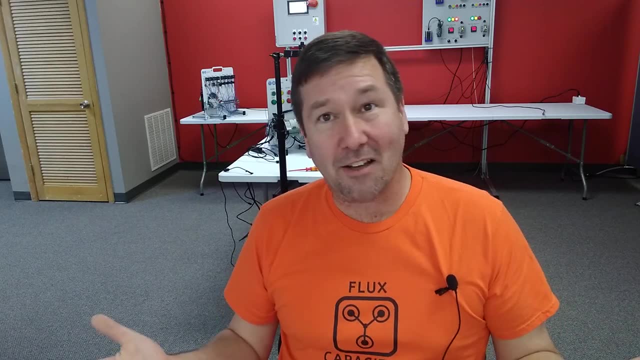 to go and talk to manufacturers and see what they're using. I mean, talk to some of the maintenance people out there and say, hey, what are you working on? or you know. if you don't know anybody in the industry, then check out LinkedIn. You can narrow it down to a location and you can, you know, ask. 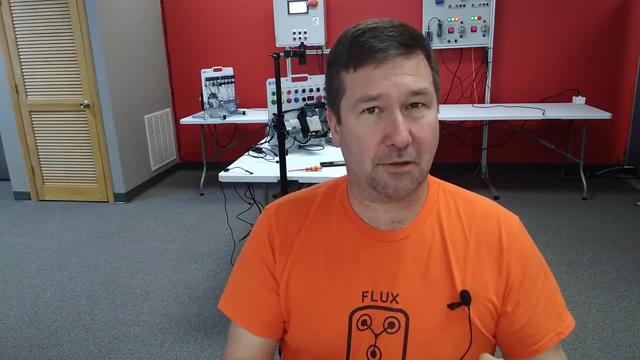 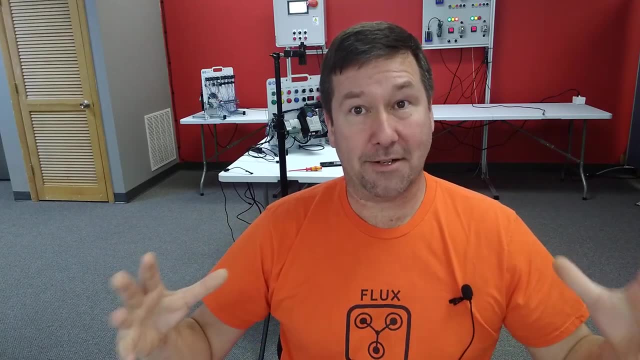 some people, And that's going to be a critical step both early on in your learning but also further down the road, Because if you learn the PLC that has these largest base in your area, then you're going to be more marketable to your area. In fact, I was 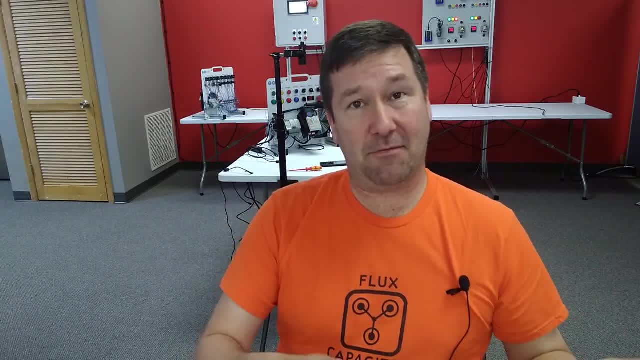 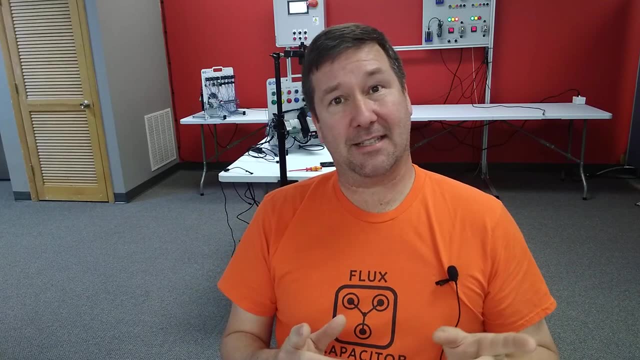 listening to a podcast the other day: Manufacturing Hub. that's Dave Griffith and Vladimir Romanov, and actually- and Vlad, he's actually another YouTuber you should check out, But they had a guest on there, Preston Hadley, and he was talking about this. that. 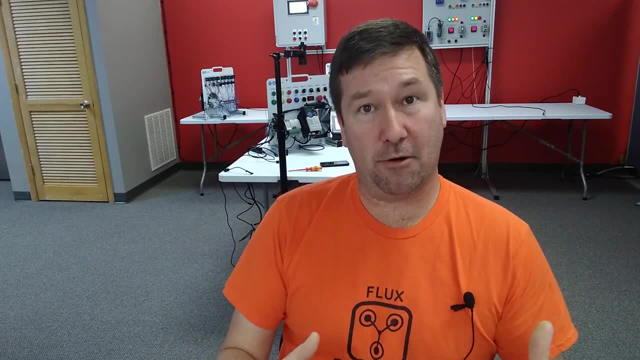 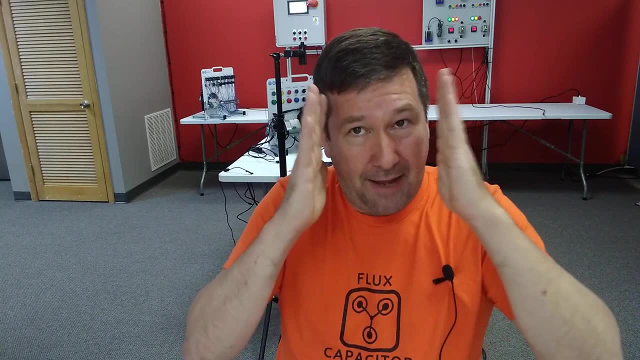 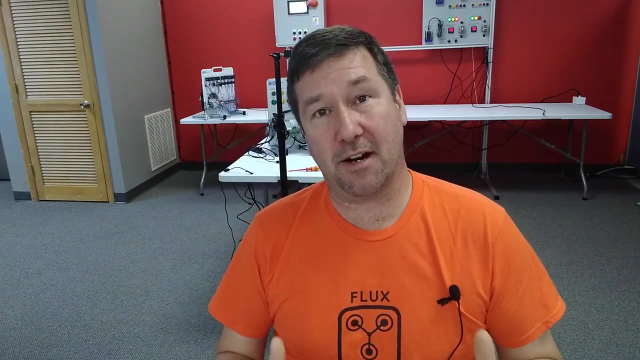 if you're looking to learn a product and how to program it with the intent of only using it on your equipment and never really having to see outside of the box, then you're probably cool learning one of, we'll say, the less popular ones in your area. to start off with, 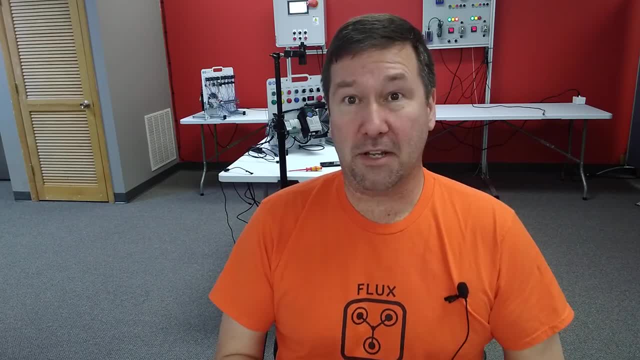 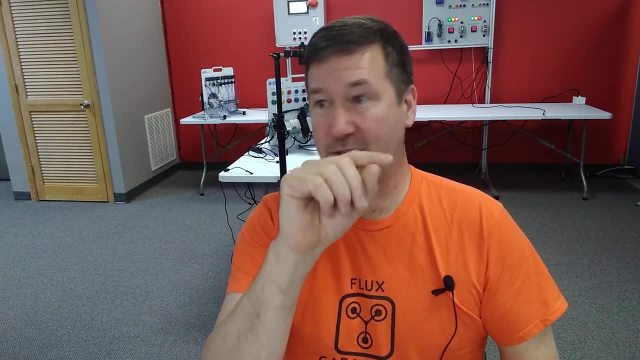 But if you're looking to improve your skills with the hope of being more marketable, job wise, then being able to write on a resume that you know how to use, whatever is the most popular in your area, is going to make you so much more marketable. 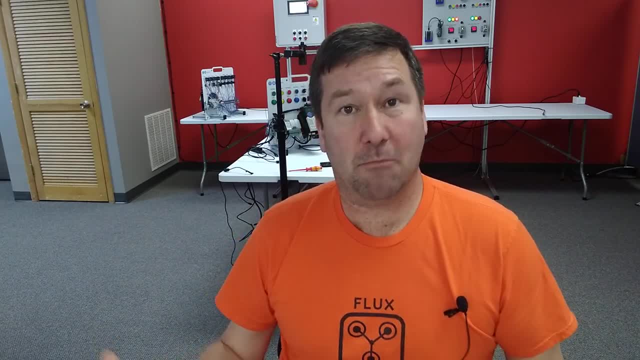 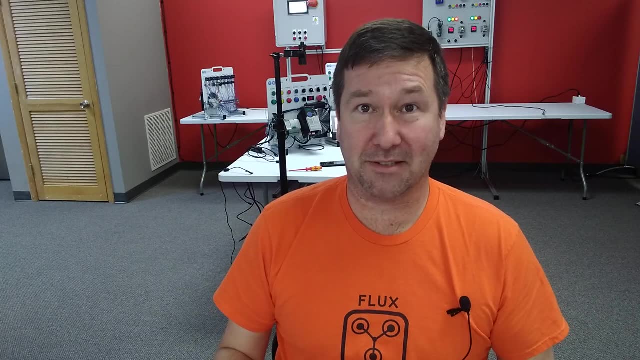 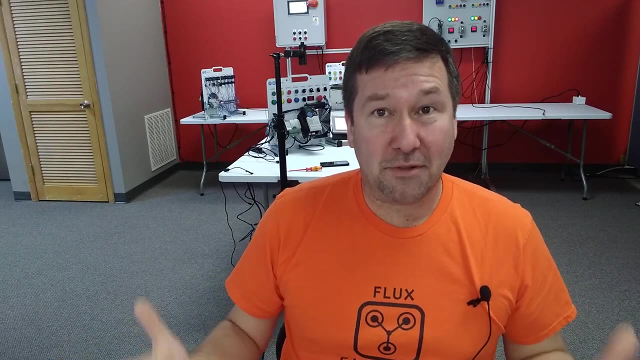 saying that, hey, I learned how to program the cheapest PLC with the free software. So that's why I think it is so important that you do select the right PLC, and I do feel the right PLC is the most popular one in your area. Now, if you've watched many of our videos, you know most of them. 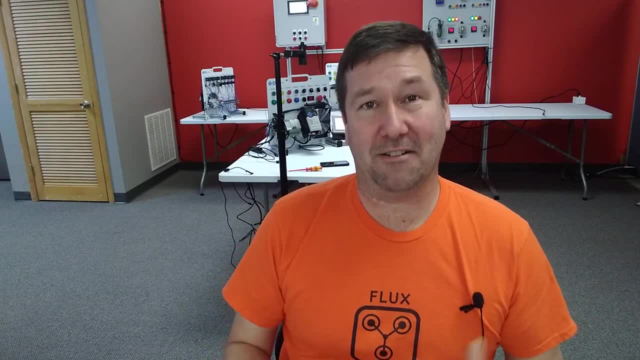 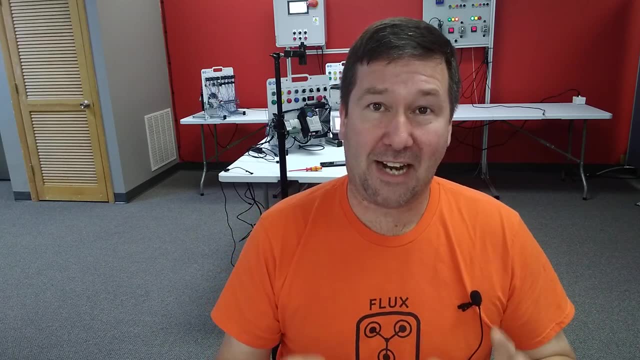 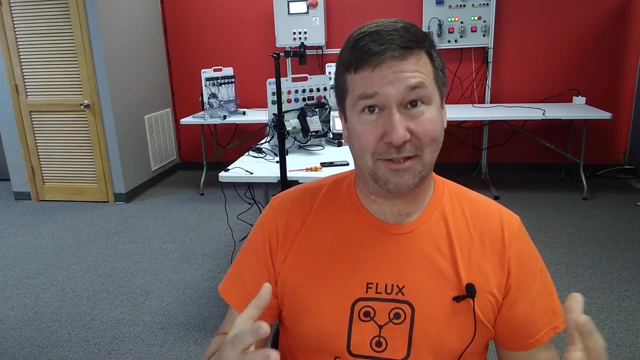 are Allen Bradley, and that's because, at least in a broad sense in the United States, Allen Bradley is the most popular. It's the one we get the most requests from and also is the one that I see put down on more job postings as a required skill. So that's why I do stick with mostly Allen Bradley. 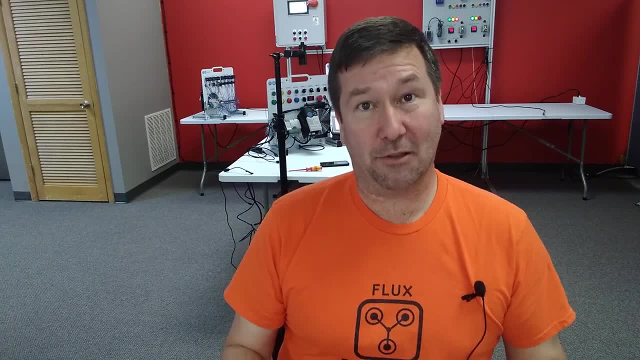 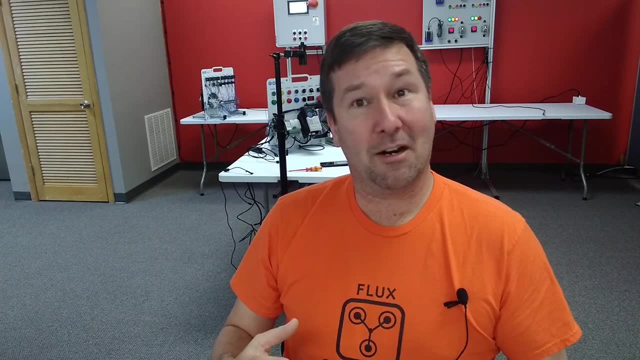 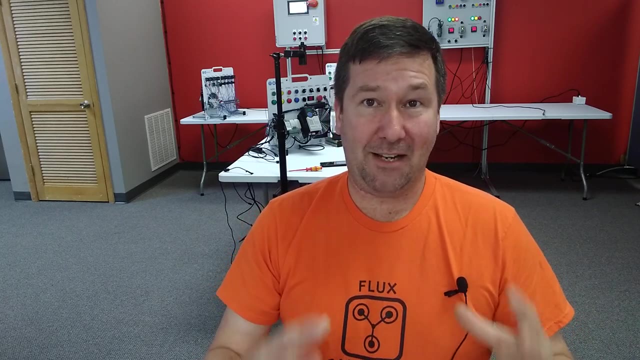 videos. In fact, we've gotten some extremely lucrative offers to use other PLCs, and as cool as that would be and really as reliable as these particular brands are, in the end, if I am not putting you in a position that makes you more marketable in. your area. I'm not putting you in a position that makes you more marketable in your area. I'm not putting you in a position that makes you more marketable in your area. I'm not putting you in a position that makes you more marketable in your area, Then I have failed and that's why we. 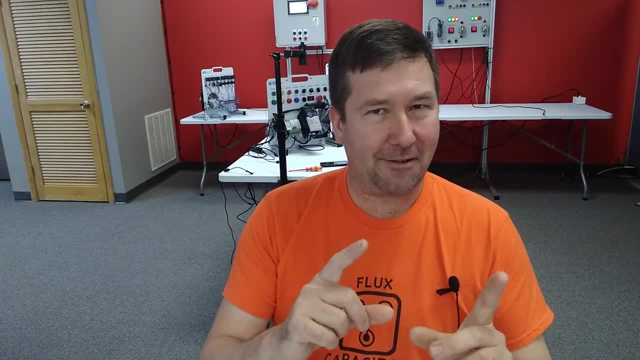 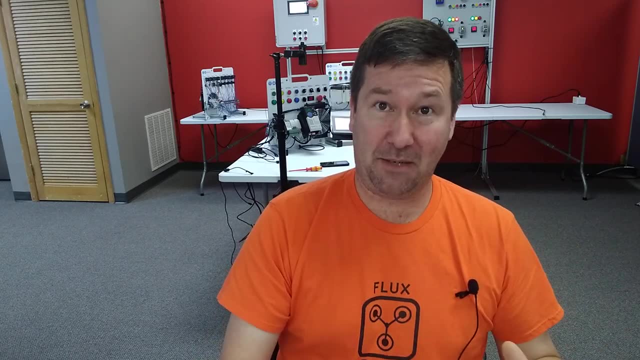 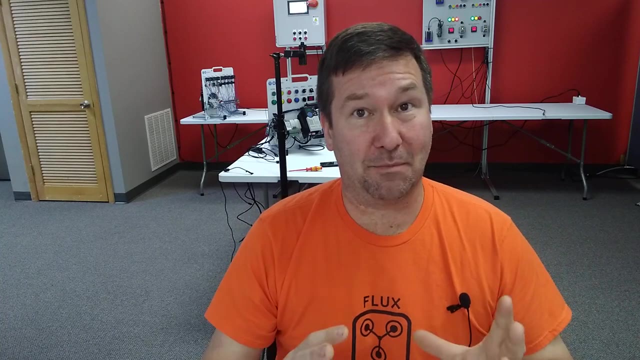 stick with the brands we do. Now there is another criteria that kind of goes along with step one that should be in your selection criteria is: if you've watched many of my videos, you know that while I believe in investing in hardware to better your skills, I don't believe and invest in the 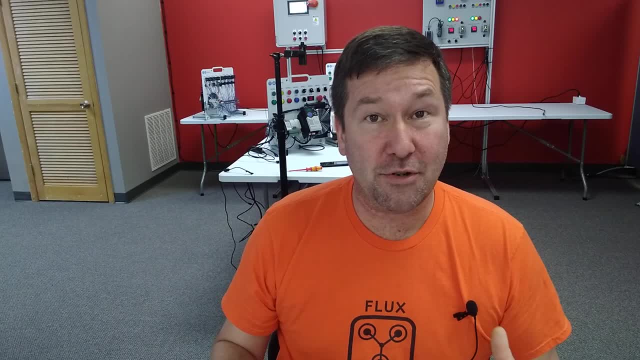 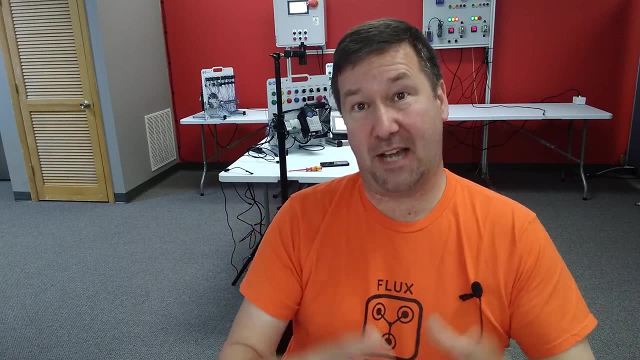 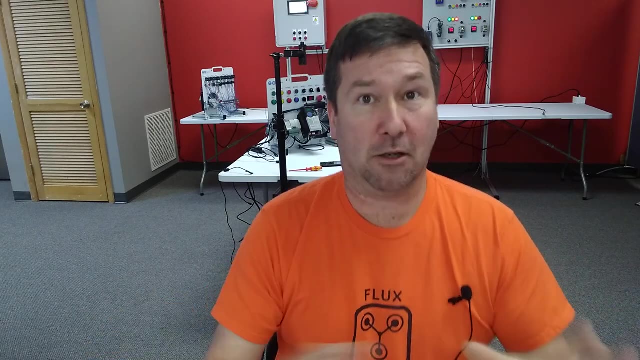 software until you need it. So the hardware you choose should have a free version of the software, free being totally free, or free being time limited or free being feature limited. and for everybody that is getting ready to type right now saying there are no free versions, Allen Bradley software. 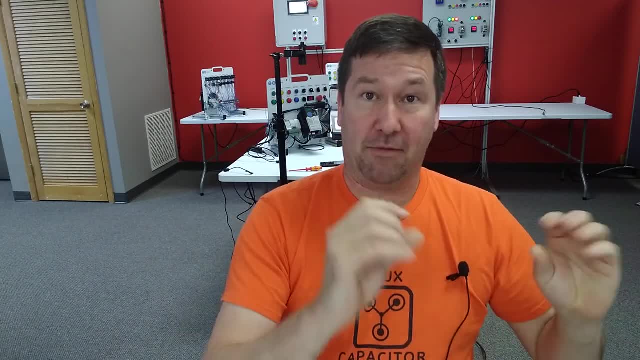 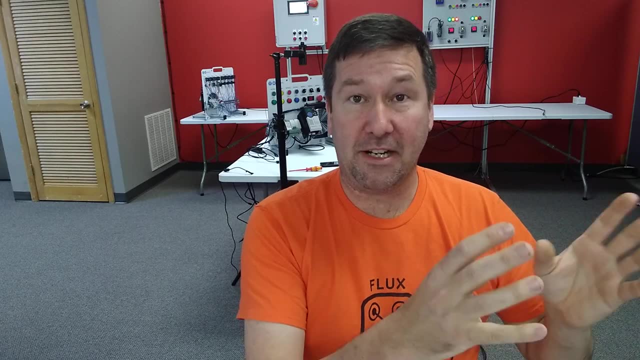 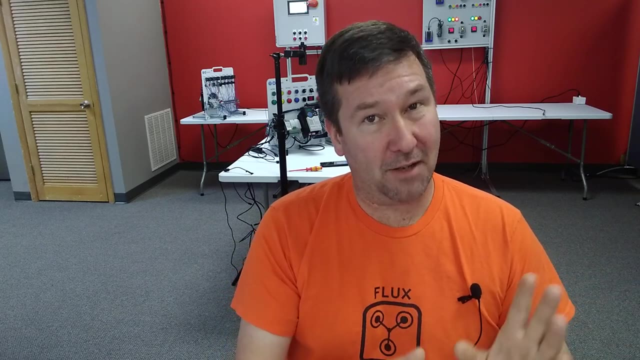 stop typing so I don't have to delete your inaccurate comments. If you're looking at the Connected Components Workbench software for the micro 800 PLC, then there is the free Connected Components Workbench standard edition and, realistically, I only recently started using the developer edition and that's because I'm getting ready to do some videos on online editing and that's the 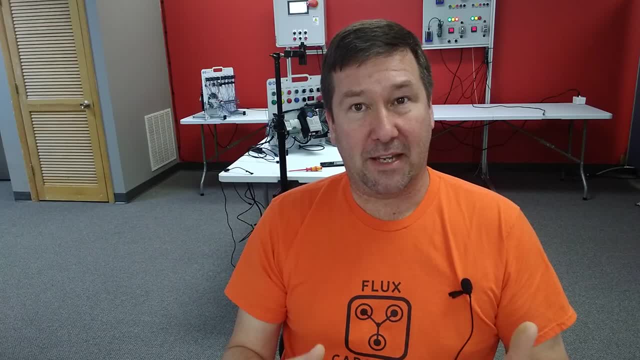 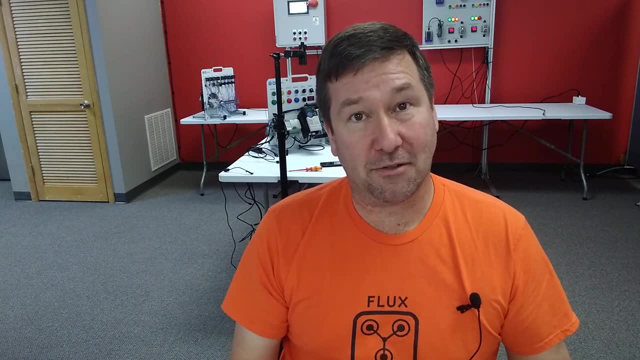 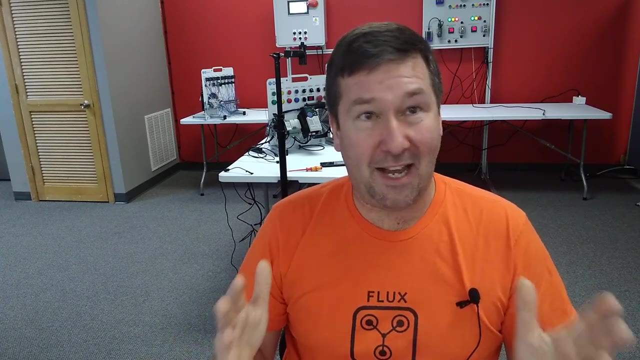 main feature that the paid version offers you. In Studio 5000 there is no free downloadable version, but all you have to do is contact your local distributor and they will give you a time limited version and chances are you can get somewhere around three to six months out of this and really 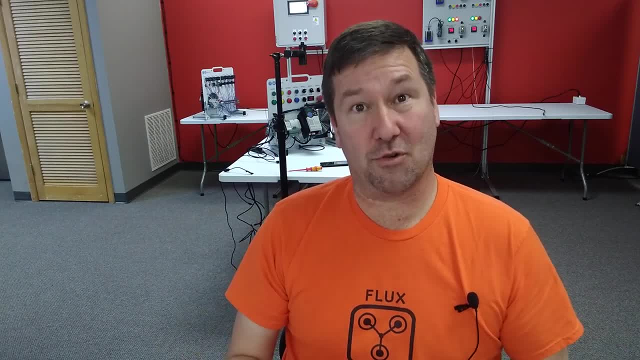 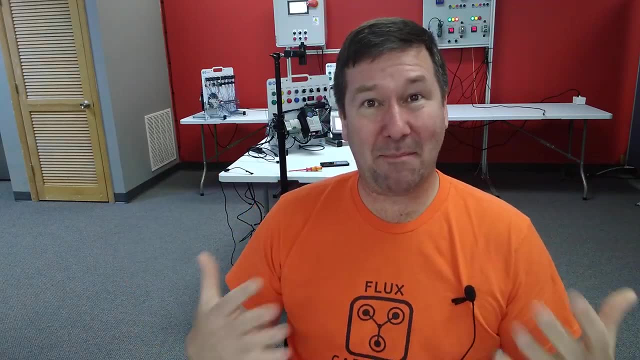 in three to six months, you'll probably have determined for sure whether you want to do this or whether you're looking for a free version of the software. So if you're looking for a free version of the software and you're like, nope, I'm done, this isn't for me and that's my main reason. 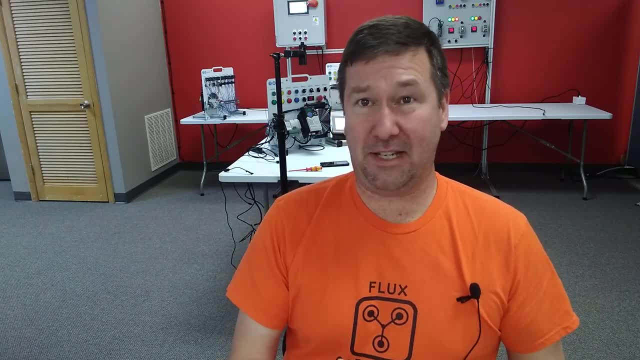 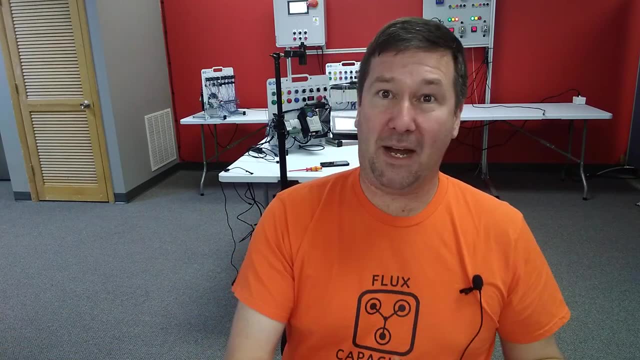 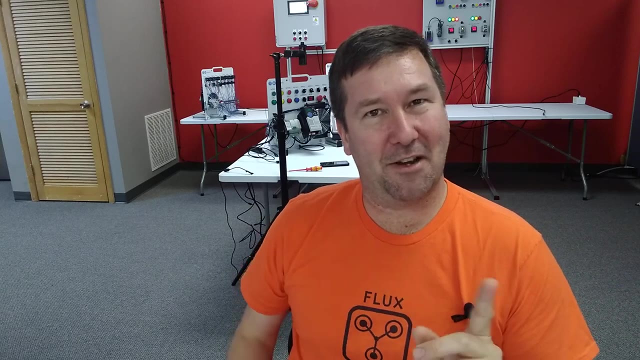 that I don't like you to buy software is because even if you buy one of our trainers, you can sell it on eBay for virtually the same price you paid for it. but if you buy software it is nearly impossible to sell, so you have lost out. Also, just because I know it'll be questioned, you don't need 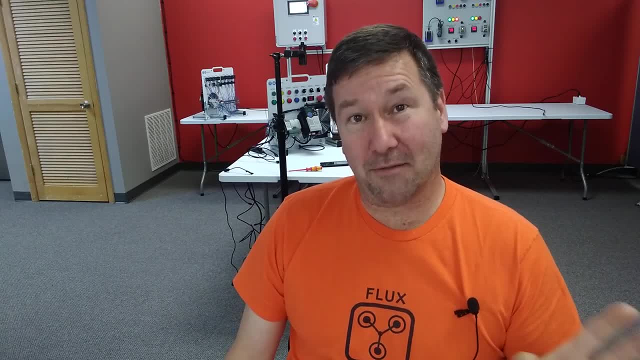 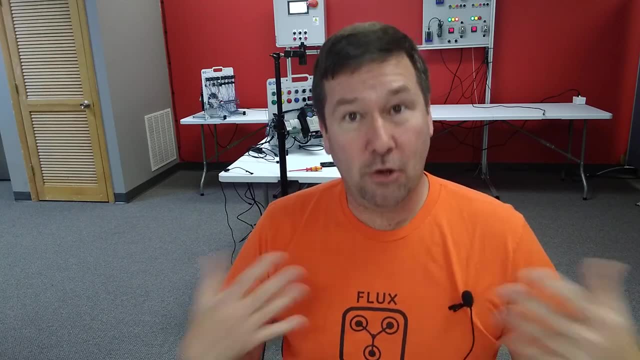 to be best friends with your Rockwell distributor to get one of these deals, because when I was starting out I got a loaner version of RSLogix 5 from my local distributor, who we had tons of bills overdue with, and they still loaned us the software, so it wasn't a buddy-buddy situation. 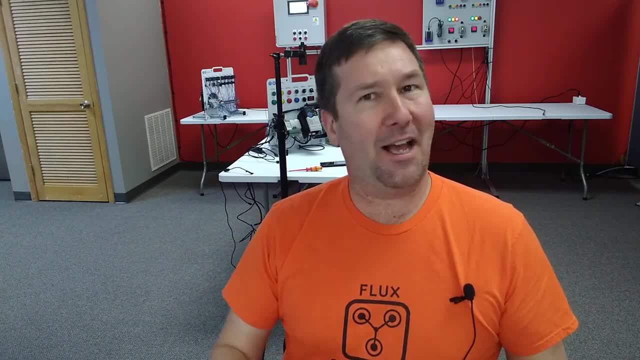 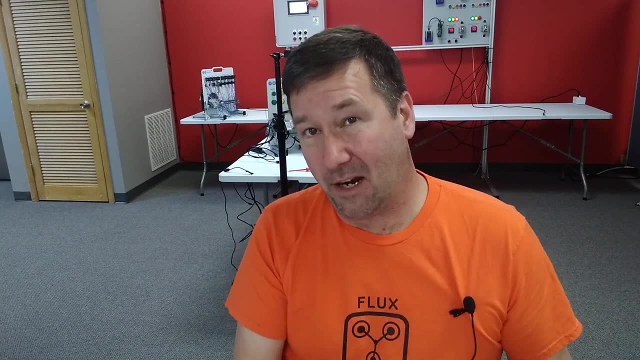 They will do this for you, so call your local distributor. I know you got to pick up the phone for this one, which is horrible, but if you will pick up the phone and you will talk to them, they also may give you some advice that may help you in your endeavors of learning or 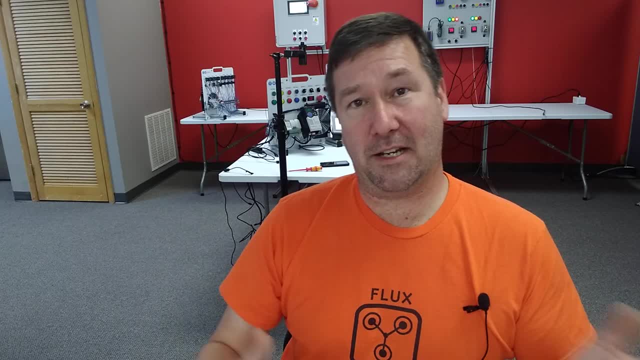 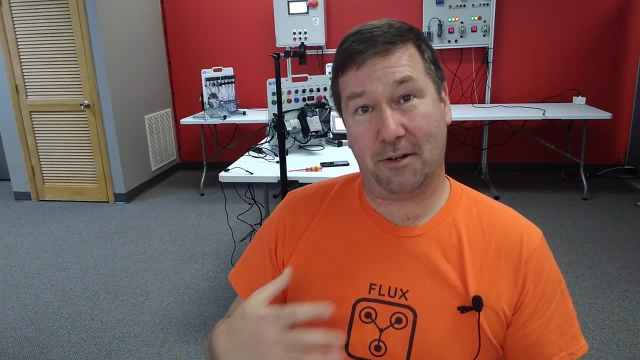 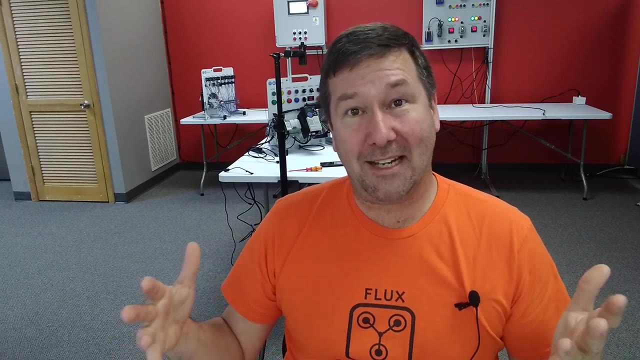 maybe they will say, hey, if you like, you could come by and we can show you some things. There is some advantages to building this relationship. but okay, that leads into what I would say is step two of learning to program PLCs, and that is installing your software. Now, notice, we have. 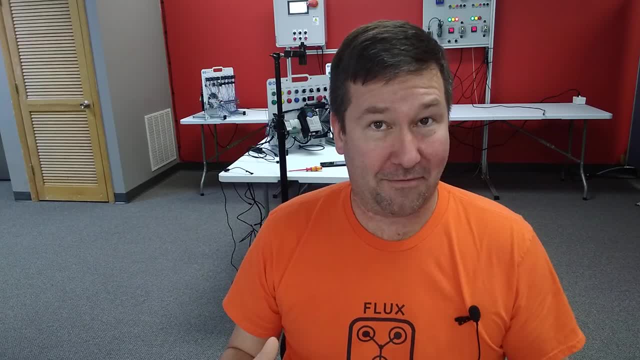 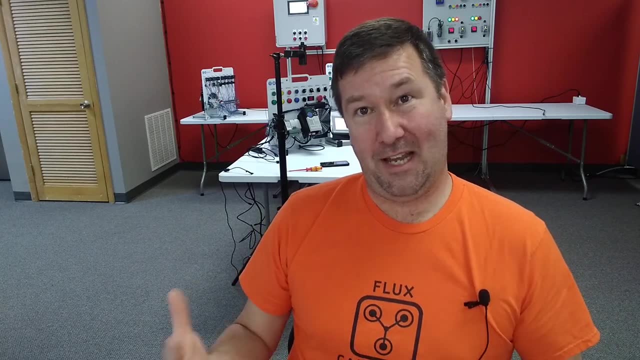 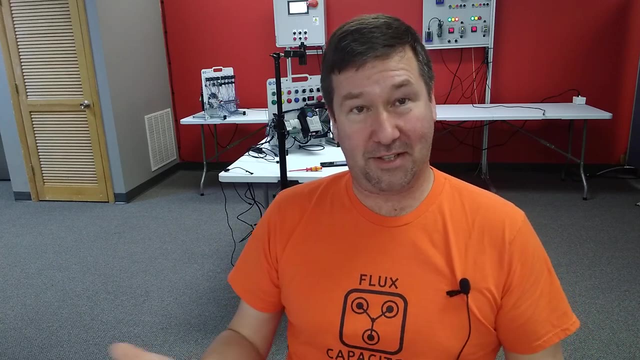 not bought any hardware yet. and there is a reason for this step, because I can't tell you the number of people I have talked to. they're like: yeah, I bought a PLC a couple years ago and now I'm trying to figure out exactly what software I need for it. I'm like man, you forked out what 500 or whatever. 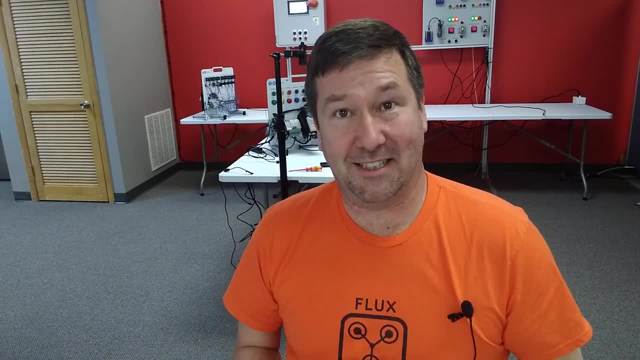 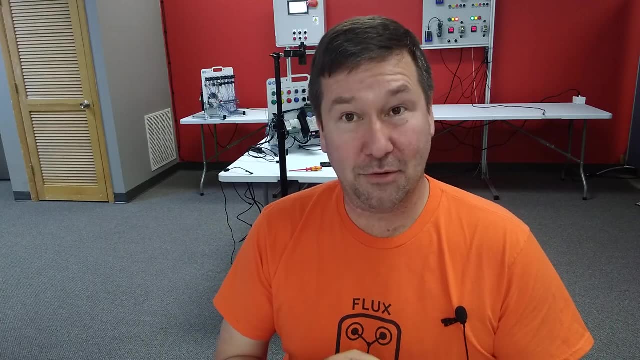 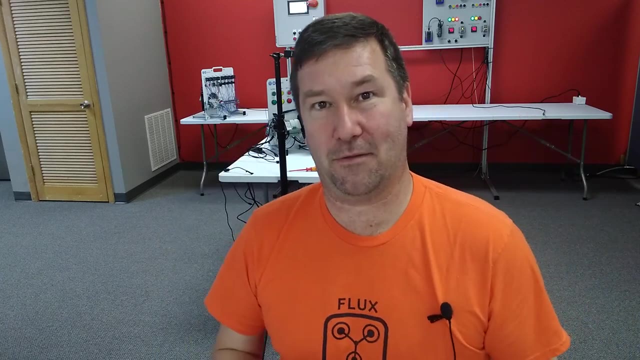 dollars a couple years ago and that box is just sitting collecting dust. So install the software. One, it's going to make sure that you're not just on a whim. Two, it's going to make sure that you don't have some activation issue or that you know you're apparently free, or you're. 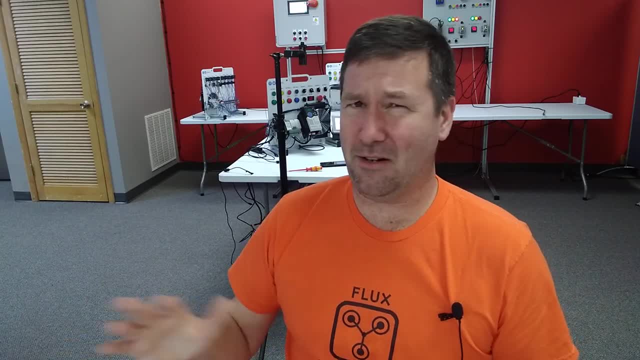 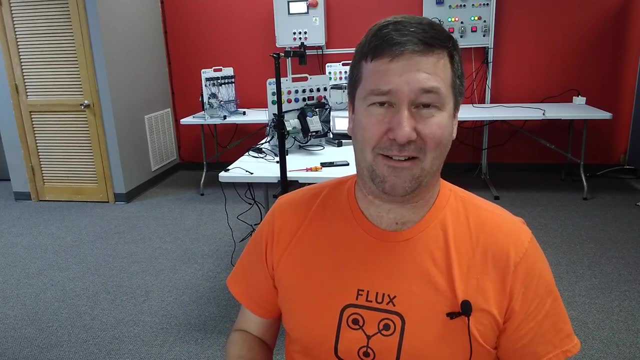 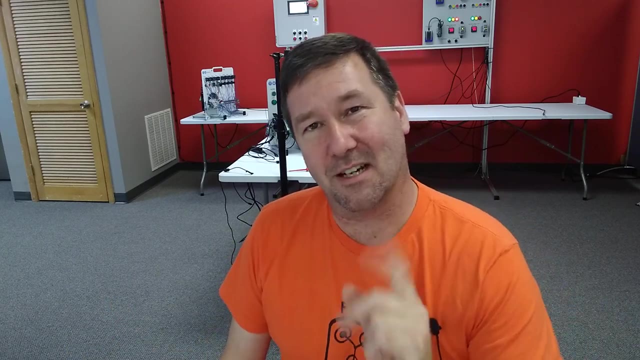 not going to be able to buy software on ebay. I mean, there are a few legit copies of software probably on ebay, but most of what's out there is pirated. I mean, I get it, you're on a budget, you know. maybe you're a student. Oh, actually I didn't touch on students enough earlier about. 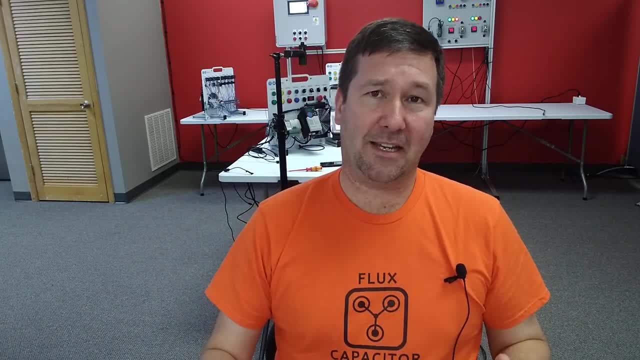 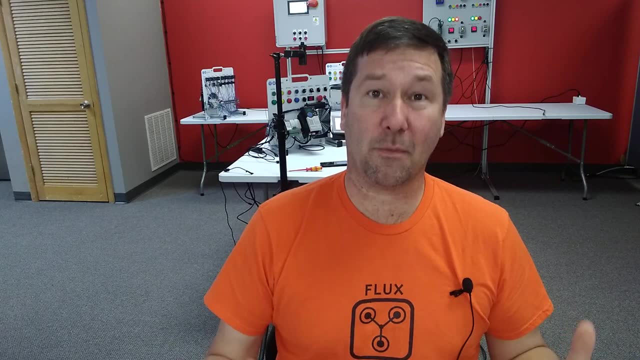 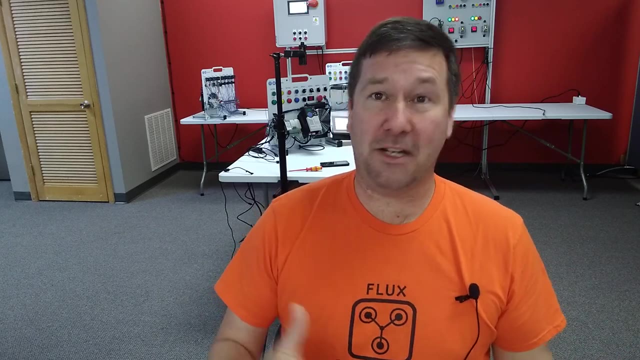 software. So colleges can get what's called the educational partner program and it allows their students to get the software for pennies, And so schools. you do need to look into that. You need to look in the educational partner program. It may be a good fit. It may not be a good fit, but it is something that is well worth reaching out to. 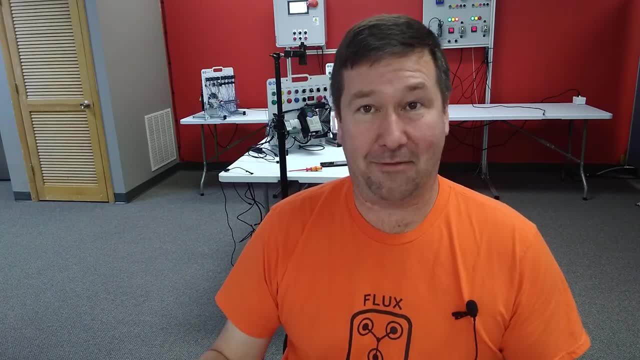 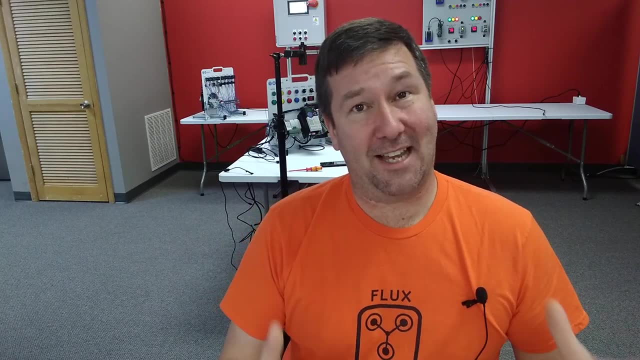 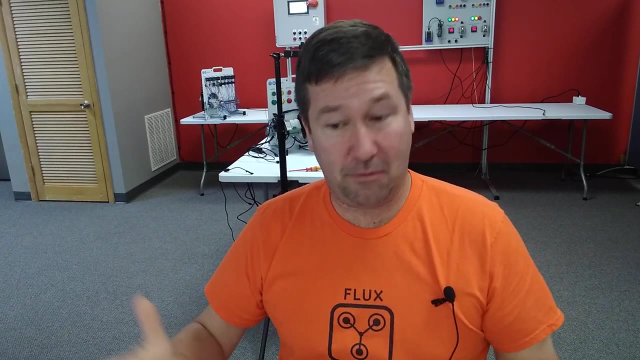 your local distributor for. But anyway, buy legit software, It's going to be worth it in the end. So then we've got our software installed, Find a set of lessons and just begin going through it And we have free lessons. I mean, if you're listening to this, I hope you know it. We have 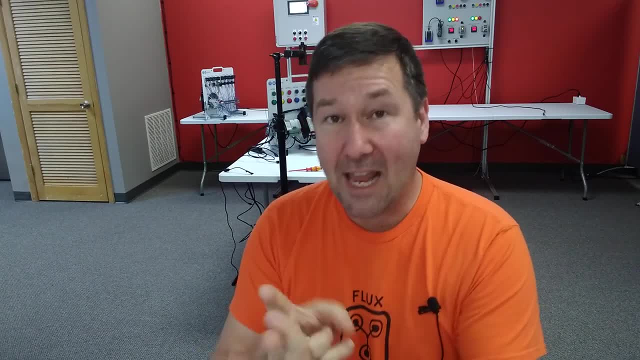 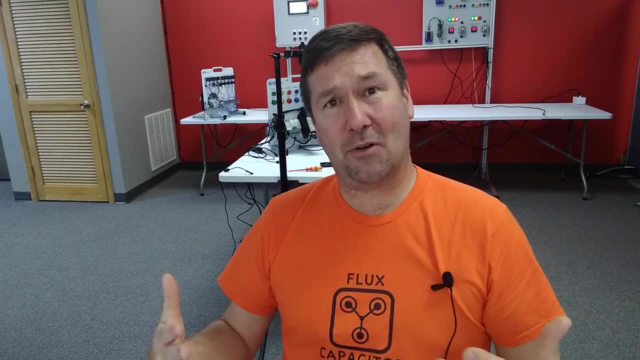 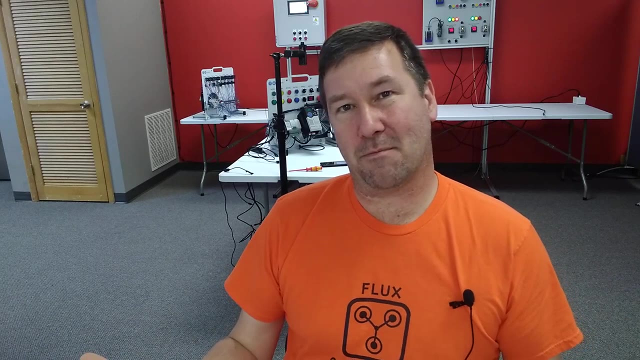 the Connected Components Workbench for the Micro 820 PLC and we have free lessons for Studio 5000 for the ControlLogix and CompactLogix PLC. So start going through them, because really you can get through several of the lessons and kind of get at least mentally a feel for it, before you ever even 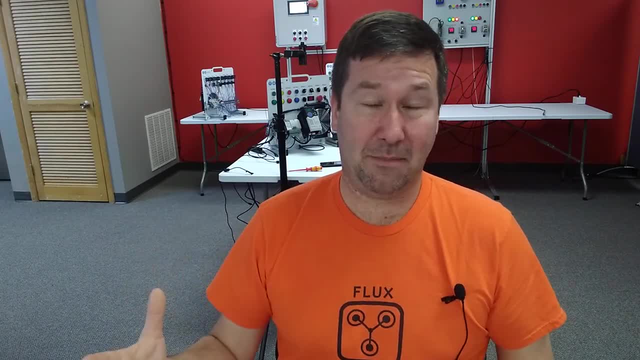 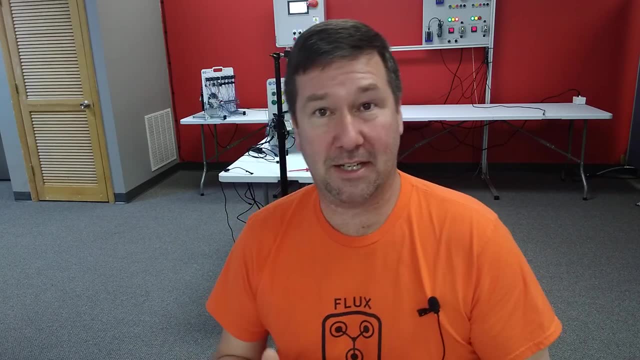 purchase hardware Now with the Connected Components Workbench. it also has a simulator, and so in that case I'd recommend going through, like the bit instruction videos, the timer videos and the counter videos before you ever even purchase hardware. So if you're listening to this, 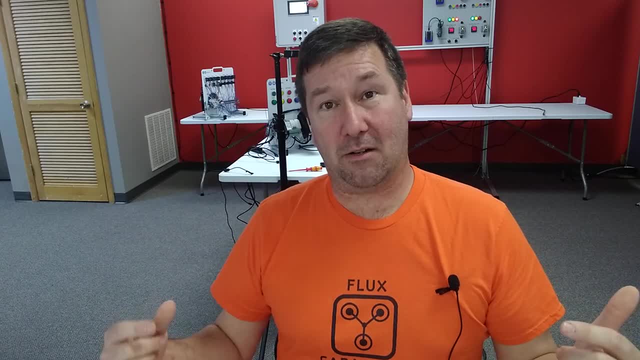 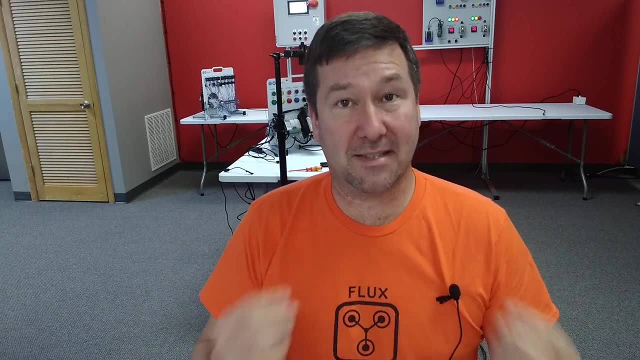 and you're thinking about investing in hardware. in fact, if you call wanting to come to the PLC lab for in-person training, that's one of the first things I'll ask you: Well, what experience do you have? If you told me zero experience, now I can get you from zero experience to troubleshooting PLCs in. 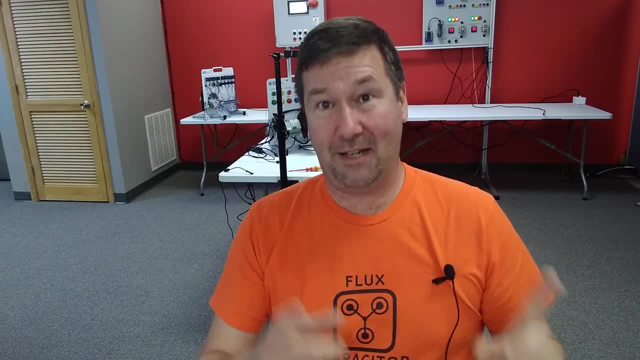 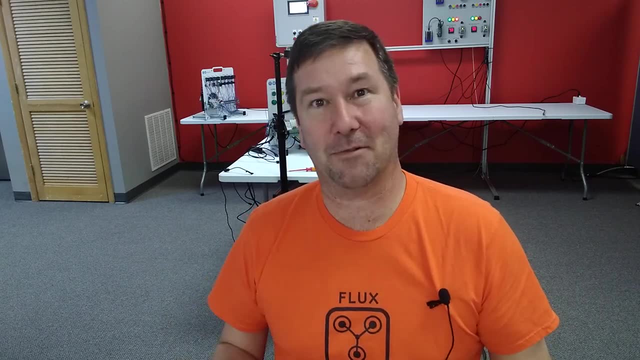 a week. But just to make sure you're really committed, I am going to make you load that software, use the simulator and go through that, just to make sure that again we're not on a whim, thinking that we're going to spend some money and magically get through that. 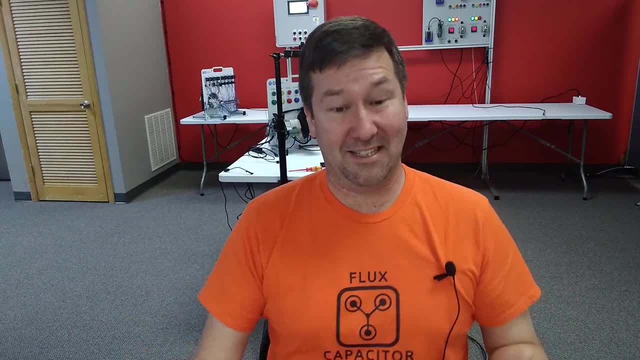 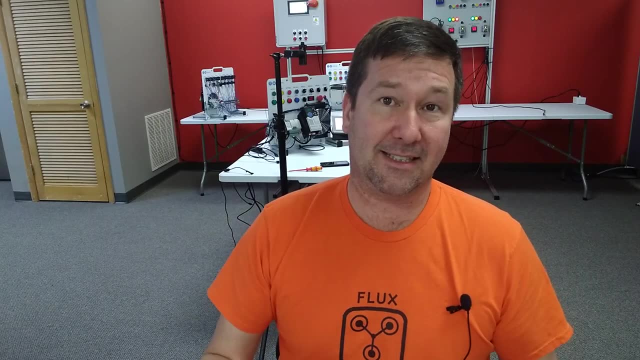 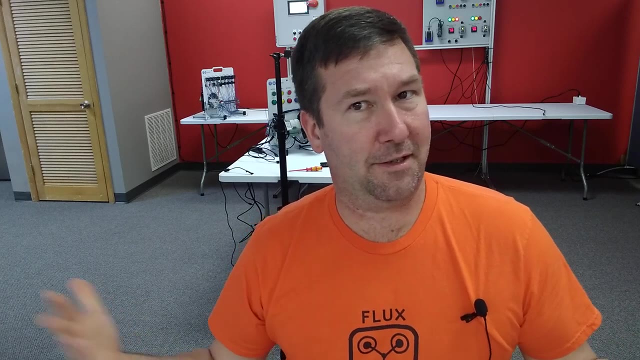 So that's what really step one and step two is about is making sure that you are committed to learning before you spend any money. And that leads us to step three, which I guess is the final step of my three steps to starting in the PLC program. I don't know, is that the title of this? 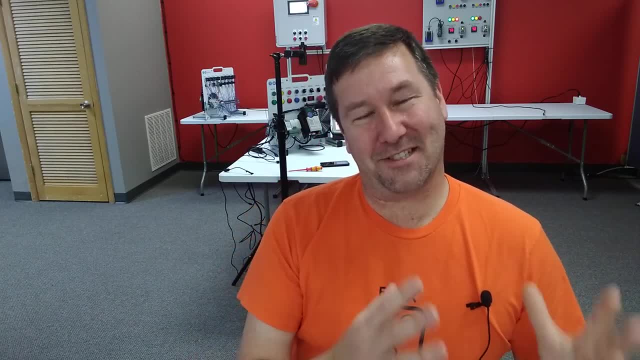 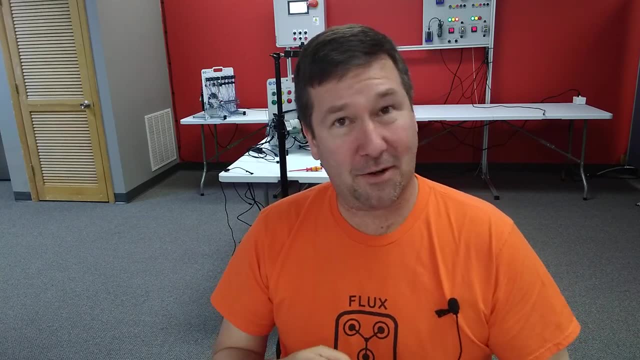 podcast. But now you're ready to purchase some hardware. We've made a really good decision on what brand we should learn. We've installed our software. we've installed our software. we've played with a little bit and figured out. okay, yeah, I am kind of interested in how this works.